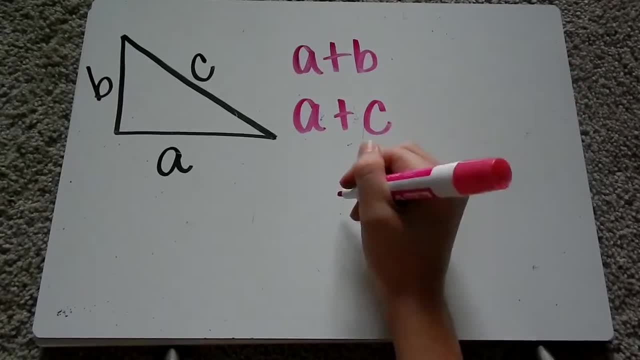 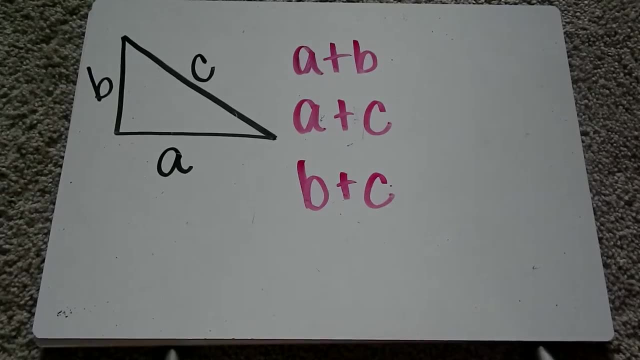 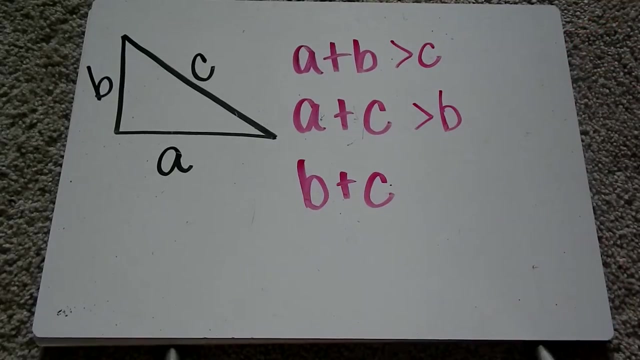 b, a plus c or b plus c. these should be greater than the third side. So a plus b must be greater than c, a plus c must be greater than b, and b plus c must be greater than a. So keep that in mind as we go through the examples. 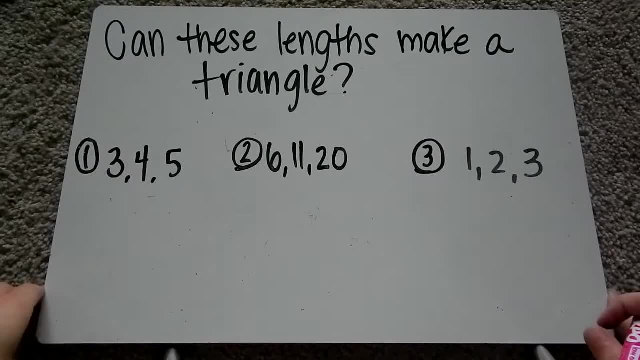 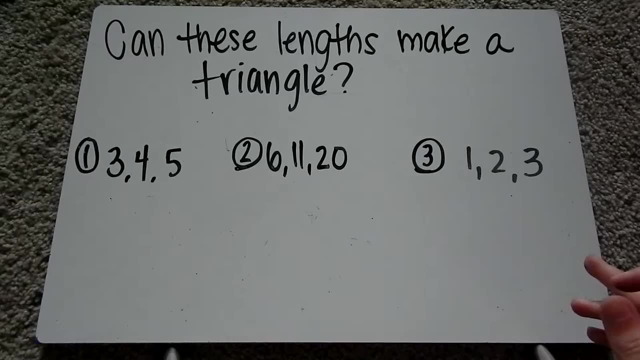 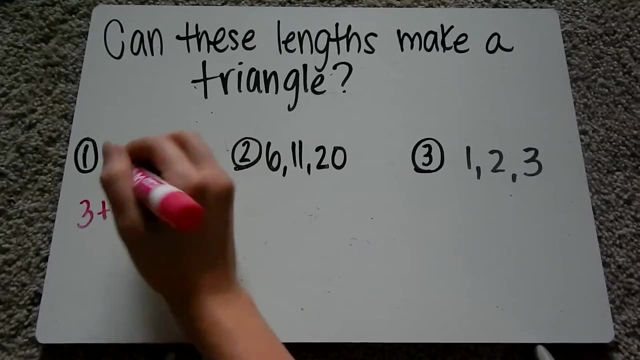 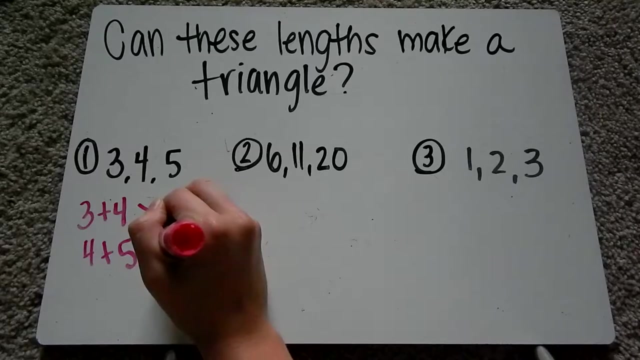 For our first set of examples. it says: can these lengths make a triangle? So we need to make sure that each pair of sides is greater than the third side. So we have: 3 plus 4 must be greater than 5,, 4 plus 5 must be greater than 3, and 3 plus 5 must be greater than. 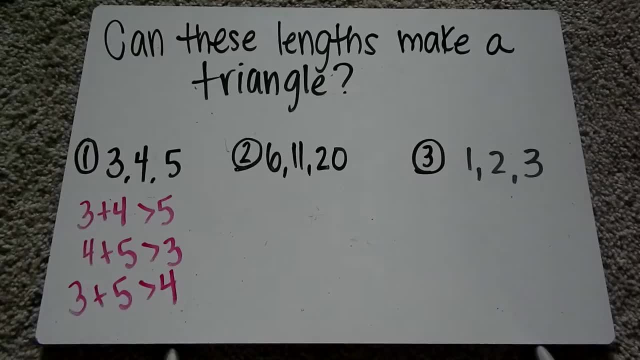 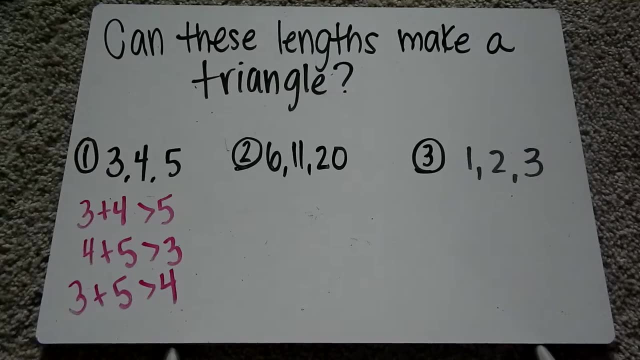 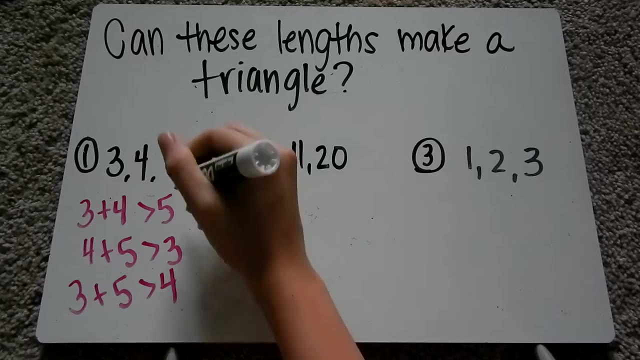 4.. So let's check these to make sure they work. So the first one there we have, 3 plus 4, is greater than 5, 3 plus 4 is 7, 7 is greater than 5, so we can check that one off, 4 plus. 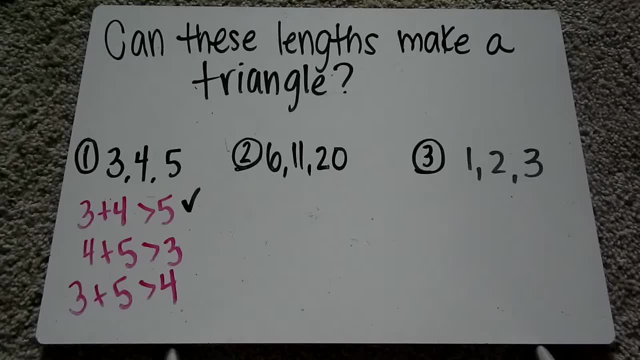 5 is greater than 3,. 4 plus 5 is 9,. 9 is definitely greater than 3, that's good, And 3 plus 5 is 8,. 8 is greater than 4.. So this one is a yes. that would be our answer Number 1. 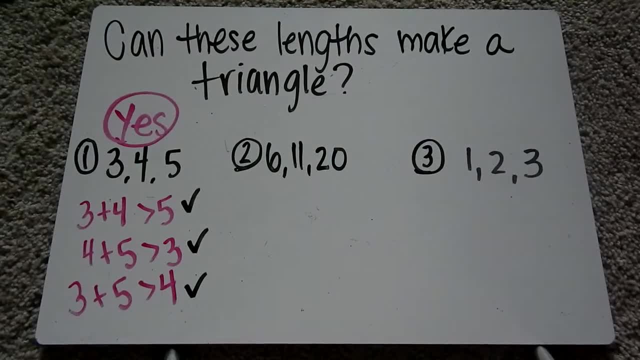 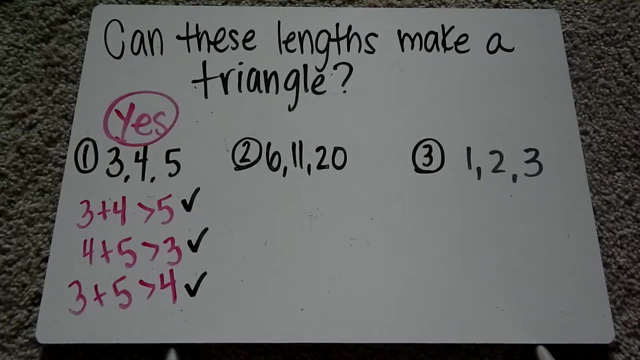 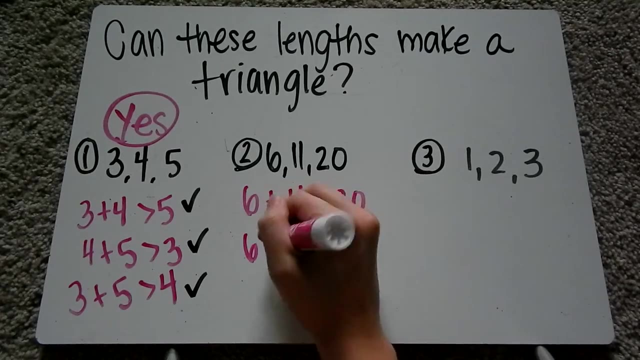 is yes, Number 2, we have 6,, 11, and 20.. So let's go ahead and see about adding these sides: 6 plus 11 must be greater than 20,. 6 plus 20 must be greater than 11, 6 plus. 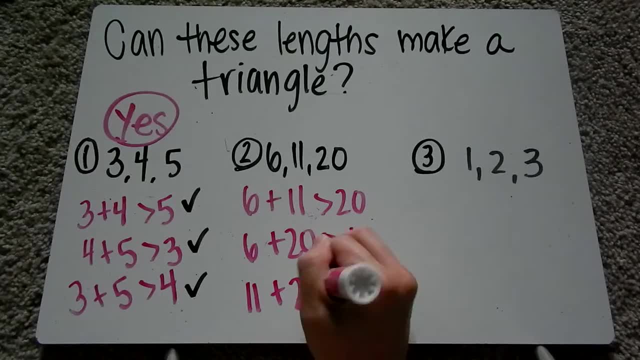 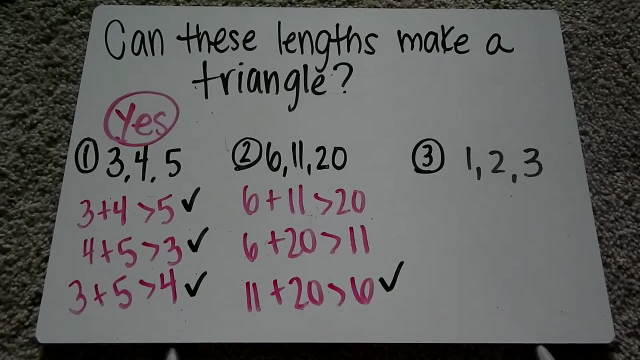 20 must be greater than 11, and 11 plus 20 must be greater than 6.. This last one is obviously true, because 11 by itself is greater than 6.. 6 plus 20 is 26,, that's greater than 11.. 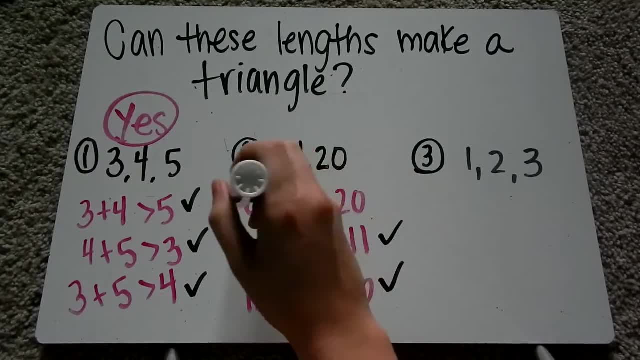 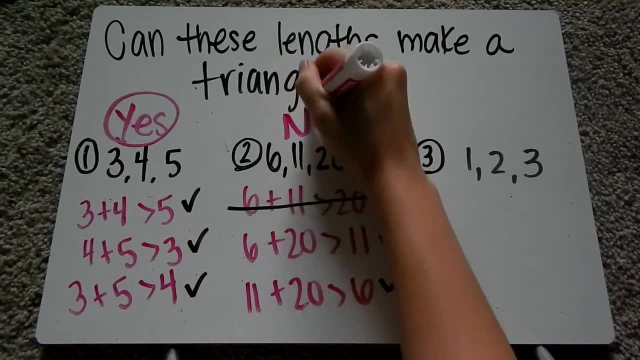 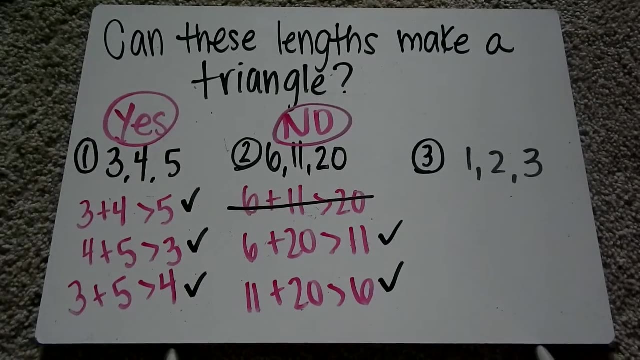 6 plus 11 is 17, that's less than 20.. So this is untrue, which means these side lengths could not make a triangle. The answer to that one is no, So we need to make sure that we're not missing out on the number of sides, So we can use the remaining two sides And the 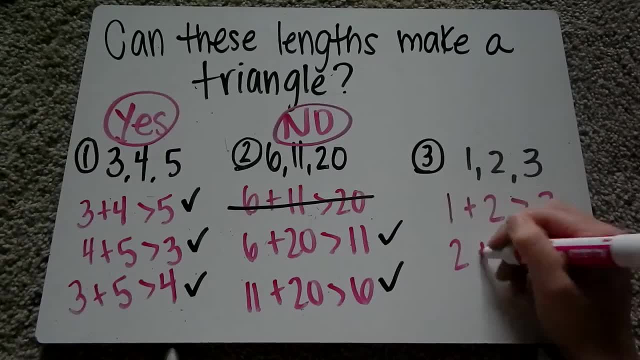 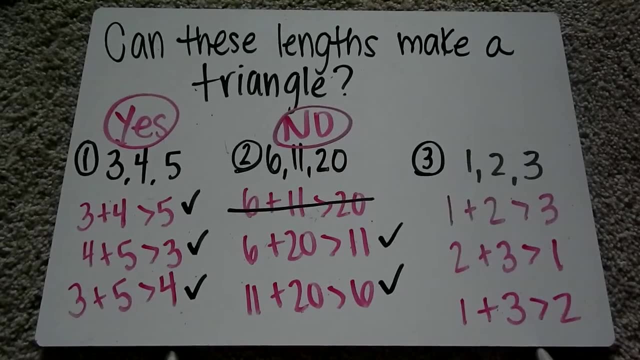 last one, number 3.. We have: 1 plus 2 must be greater than 3,, 2 plus 3 must be greater than 1, and 1 plus 3 must be greater than 2.. So, going down the line there, we have 1. 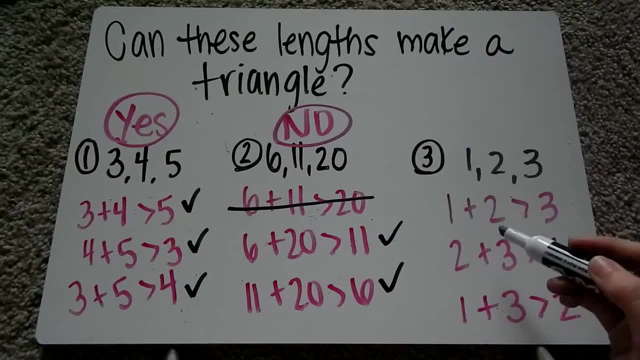 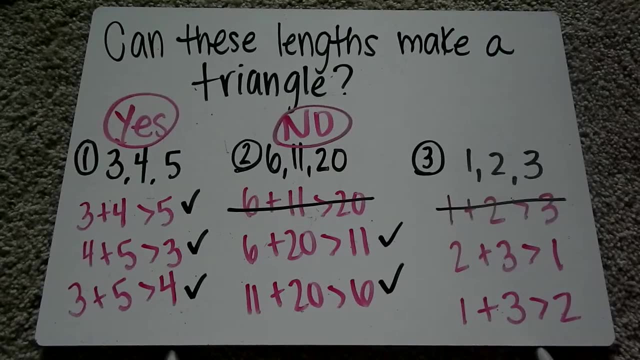 plus 2 is greater than 3.. 1 plus 2 is 3.. 3 is not greater than 3,. 3 is equal to 3, so that's wrong and this one could not form a triangle, so that is a no there. 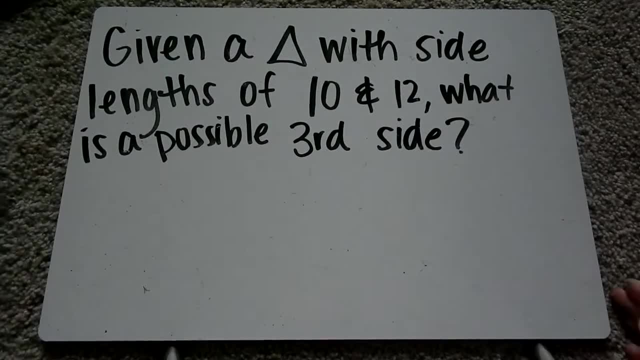 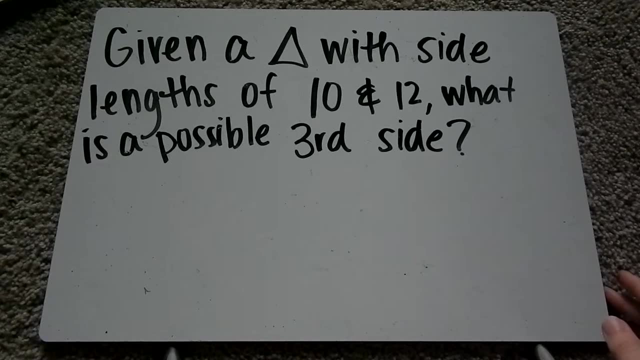 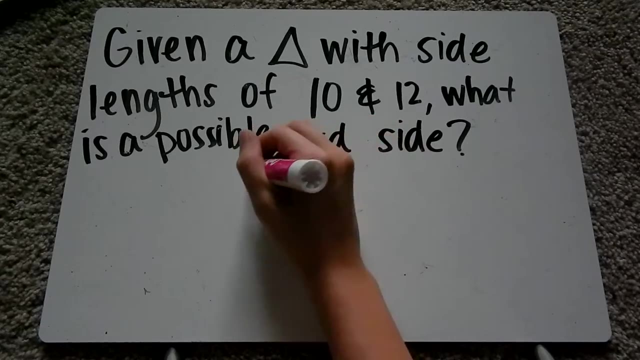 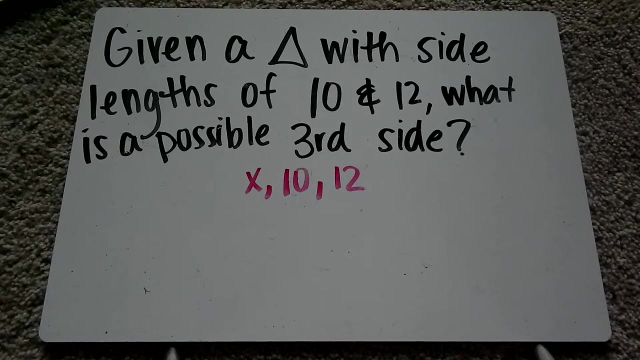 Moving on to our next example. This example says: given a triangle with side lengths of 10 and 12, what is a possible third side? So let's go ahead and list out our three sides. We have some side x, We have 10 and 12.. So I'm going to list out the three things that need to be. 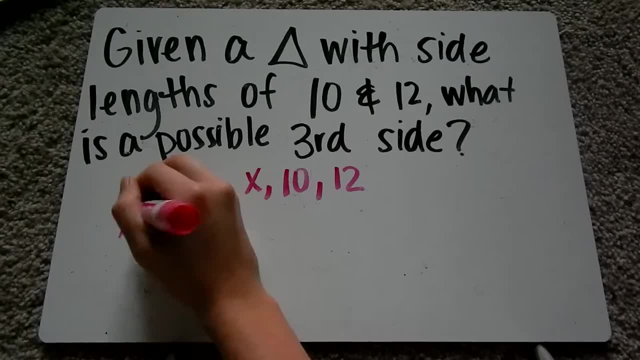 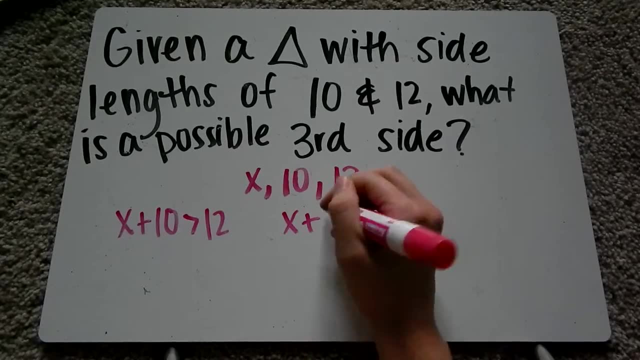 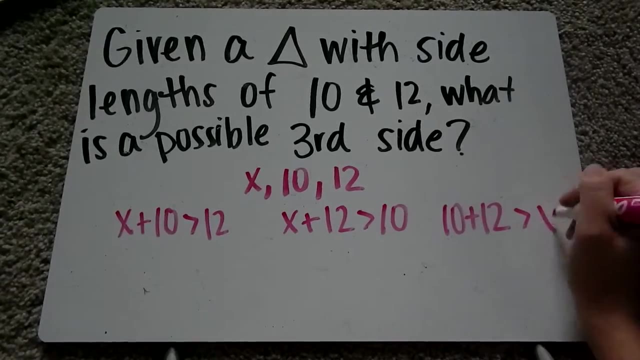 true for this to be a triangle. So x plus 10 must be greater than 12.. Then we have: x plus 12 must be greater than 10, and 10 plus 12 must be greater than x. Those are the three things we have to prove. 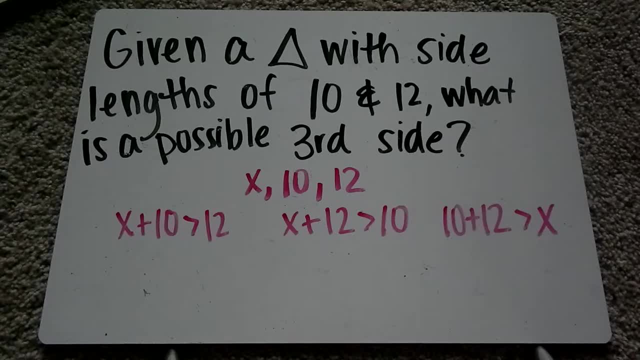 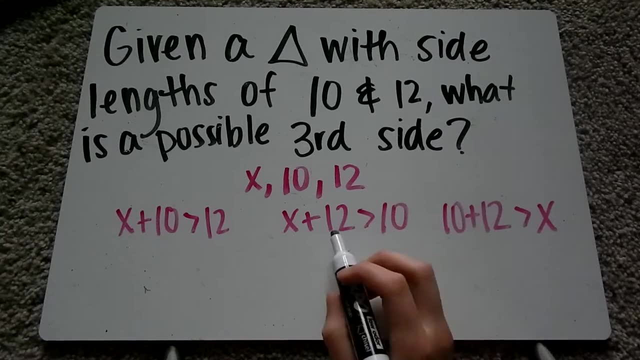 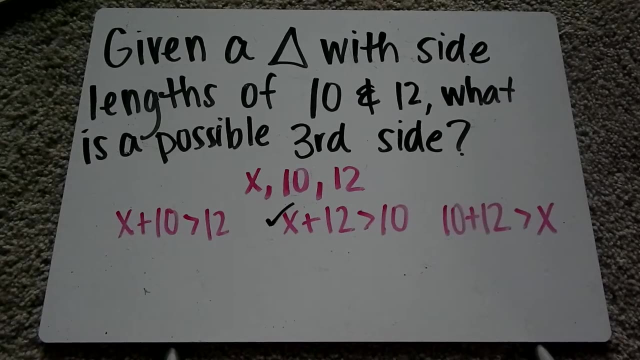 To make sure we have a triangle. Those three things have to be true. Now, if you look at the middle equation, or inequality there, x plus 12 is greater than 10.. 12 is already greater than 10, so this is true regardless. So this is already a check. We don't have to do anything else to that. 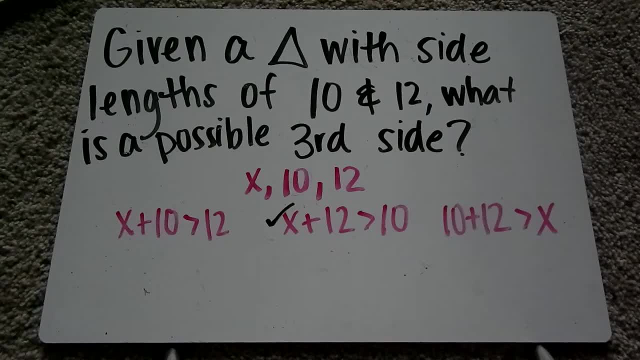 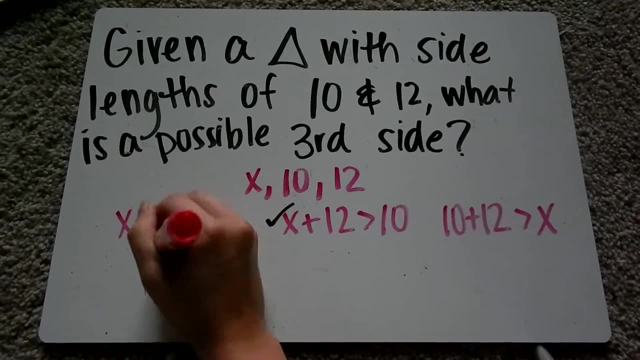 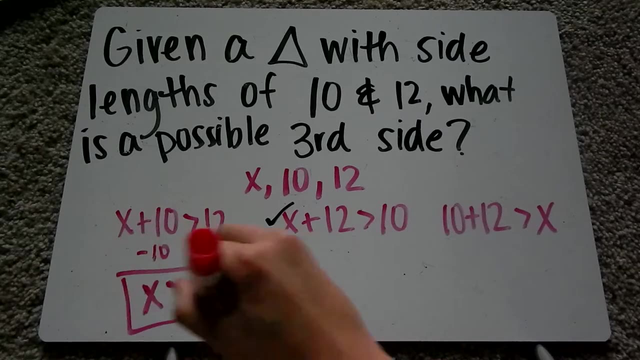 Now the first inequality: x plus 10 is greater than 12.. Well, let's figure out. try to figure out what x is by solving. So we subtract 10 from each side and x must be greater than 2.. So x has to be a number greater than 2..